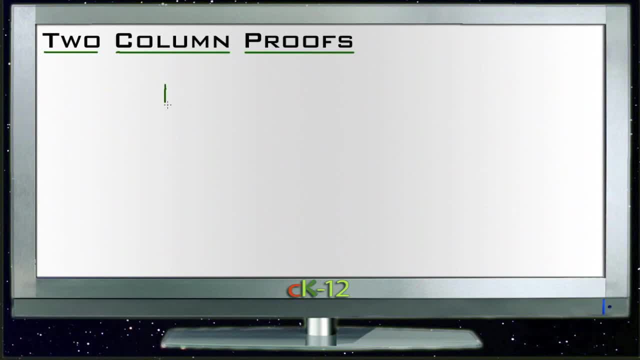 overview. what you're going to do is take your piece of paper and make two columns in it- hence the name- two column proofs. And you're going to make one column marked statement And then the other column marked reason, And just like we did kind of in the last lesson- 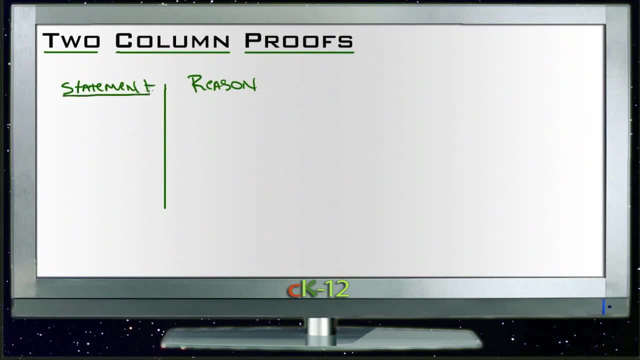 there, the statement is going to be sort of the step or the action that takes you one step closer to going from your initial state or your initial position to your final position, And the reason will be the proof or the proof of the statement, And then you're going to 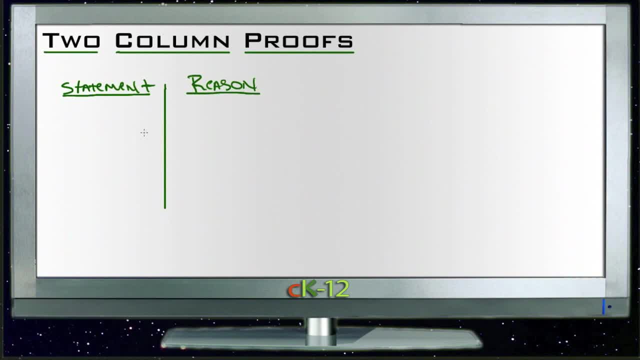 use a postulate that justifies why you're doing that at each step of the way. Be sure, along the way, that you number each step so that it's easy to keep track. Recognize that if you have, say, two statements in a row that are the subtraction property of equality. 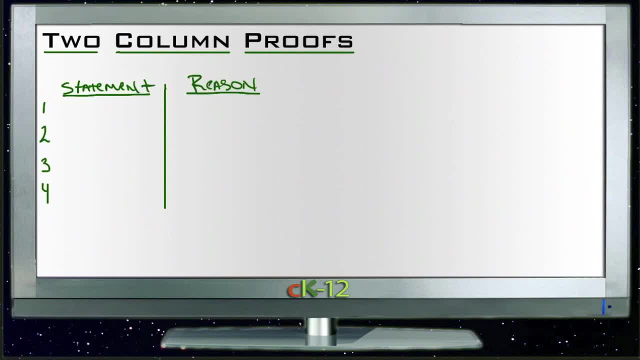 you can do them both at once and just call it subtraction property of equality. You don't have to have a separate step just for that. It's a good idea often to draw a picture and mark it with information, And then you're going to take your piece of paper and you're going to 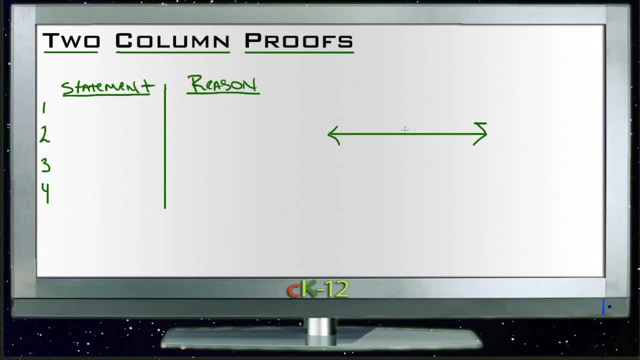 mark it with information If you have. you know a statement that says something about two points on a line. draw the line and draw the two points, because it's easier for you and for the person going along with your proof to keep track of what you're saying. Remember. 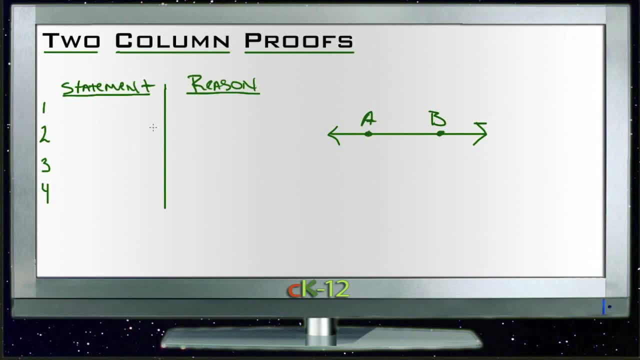 that you have to have a reason for every statement that you make. The order of the statement isn't necessarily important, as long as the order makes logical sense. I mean you can't go straight from you know, A plus 20 equals C to, for example, A plus 20 equals A plus. 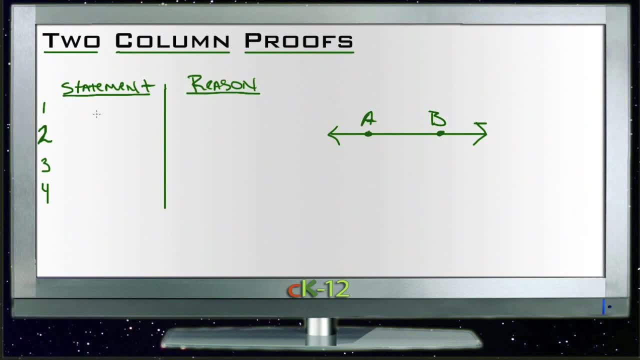 4A minus 80 equals 7C, or something You can't. You have to make sure that your order of operations follows clearly and that it's a logical progression, And then make sure that you are using, for your reasons- you're using- definitions, postulates, properties, and you can if you prove something. 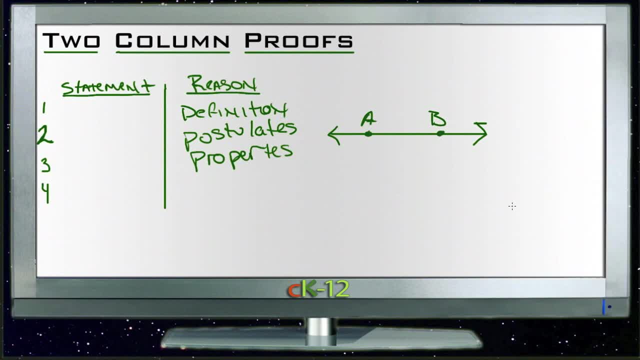 at one point, then you can go ahead and use it farther along in your. if you prove something at one point, you can go ahead and use it farther along in your two-column proof. but make sure you have to prove it, or make sure you have proven it first, before you rely on.